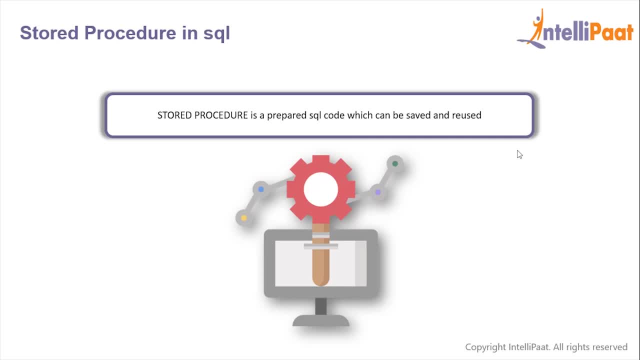 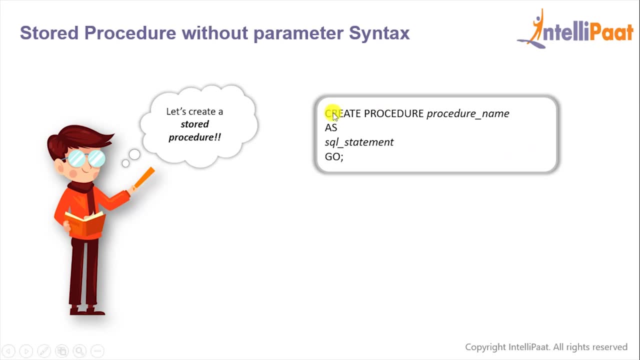 over and over again. we can save it as a stored procedure and then just call it whenever we want. Now let's have a look at the syntax of the stored procedure. So we'll give the keywords create procedure and then give the procedure name. After that we'll give the. 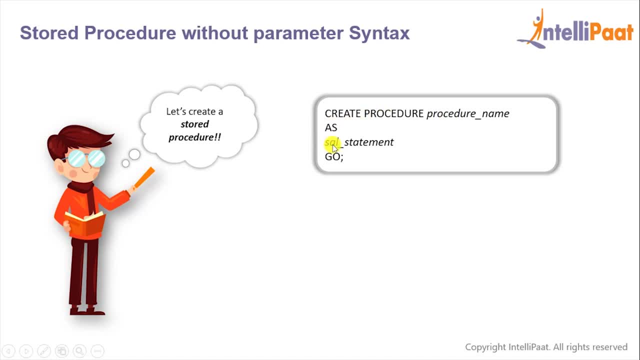 keyword as and then give the SQL statement for which we need to create the procedure, and we'll end the procedure with the go keyword. Now, after we create a procedure, we need to execute it. So this is the syntax to execute the procedure: We'll type exec and then give 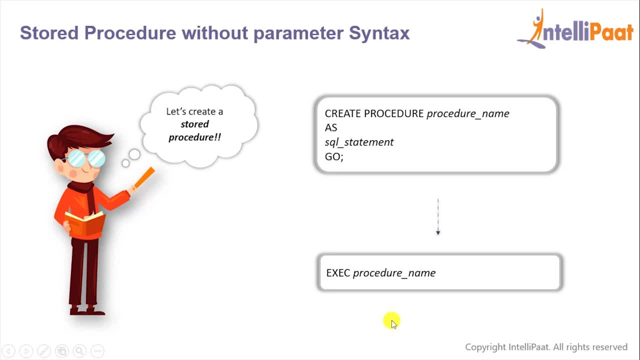 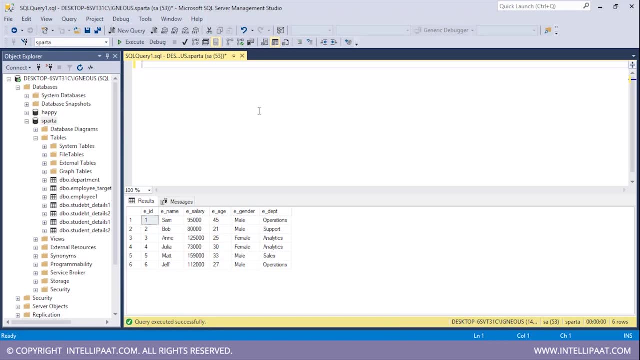 the name of the procedure which is to be executed. So let's go to SQL Server And work with some procedures. So now I want to create a procedure which would help me to easily access this eh column from the employee table. So I'll type create procedure and then 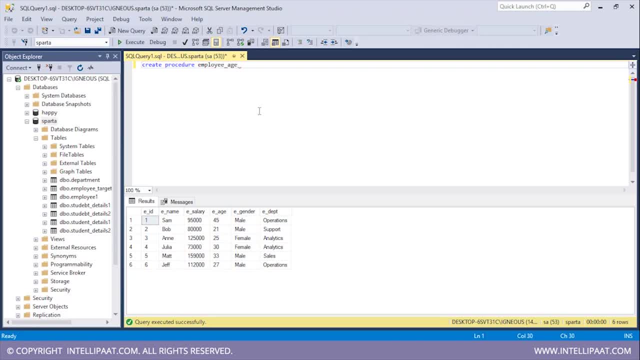 I'll give the name of the procedure, which would be employee age. I'll type as and then give the SQL statement which would help me to access this eh column. That would be select eh from the name of the table is employee. Okay, And then I'll give the go keyword. Now I'll hit execute. Right, So we see that we have. 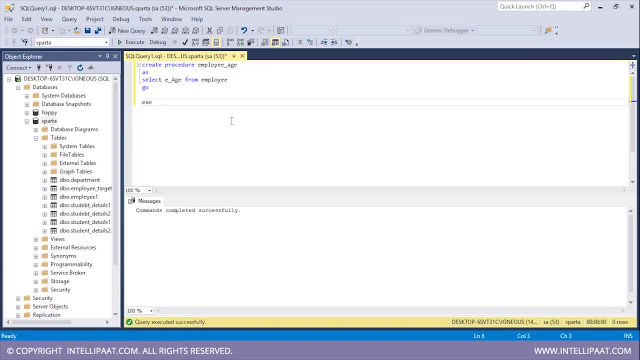 successfully created the employee age procedure. Now I will use the exec keyword and then call this procedure. So the name of the procedure is employee age. I'll select this line, I'll hit execute Right. So with this employee age procedure, we can easily access the eh. 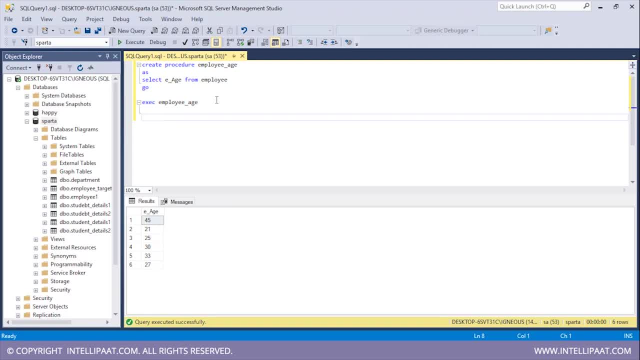 column from the employee table. Now, similarly, I'll create another procedure which would help me to access all of the records From the employee table: create procedure and I'll name this procedure as employee details. I'll follow it up with the ask keyword and then give the SQL statement which would help. 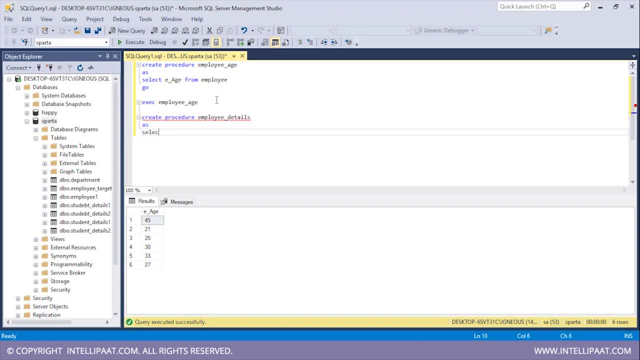 me to access all of the records from the employee table. Select start from employee. And again, I'll finish this procedure off with the go keyword. I'll select all of this, I'll hit execute. So again, we have successfully created the employee details procedure. Now to call this procedure. 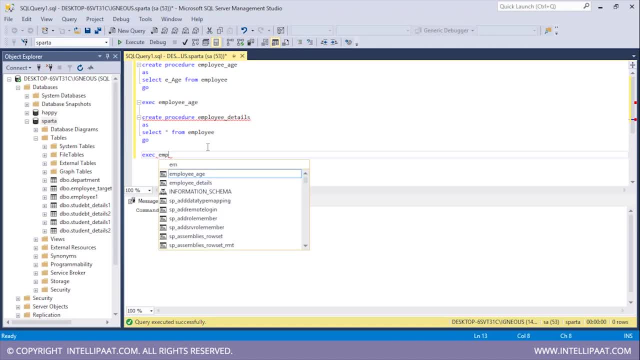 I'll use the exec command and then passing the name of the procedure, which is employee details, So I'll select this. I'll hit execute Right. So, with the help of employee details procedure, we can easily access all of the columns and all of the records from this employee. 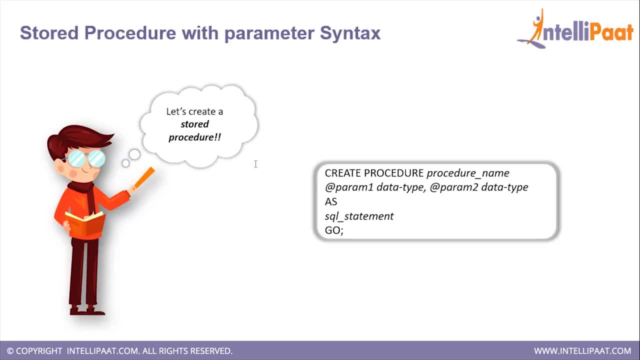 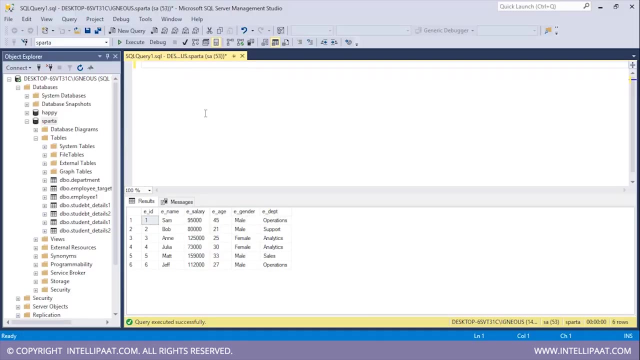 table. Now we can also pass parameters to the procedure, So the syntax for this is just slightly different. Here, after giving the procedure name, we follow it up with the list of parameters and their corresponding data types. So let's create a procedure with a parameter now. So now I'll create a. 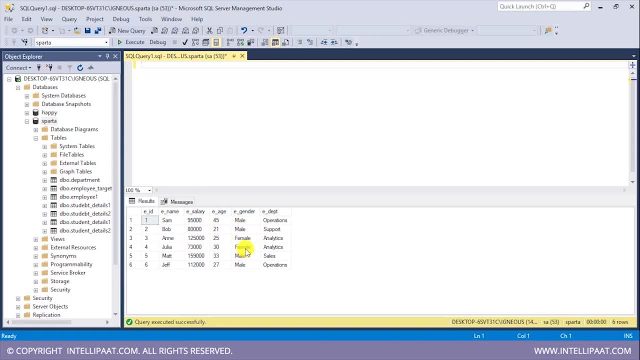 procedure which would help me to access the male employees and the female employees separately from this employee table. Create procedure and I'll name this procedure to be employee gender. After this, I will pass in the parameter, So the name of the parameter would be gender. 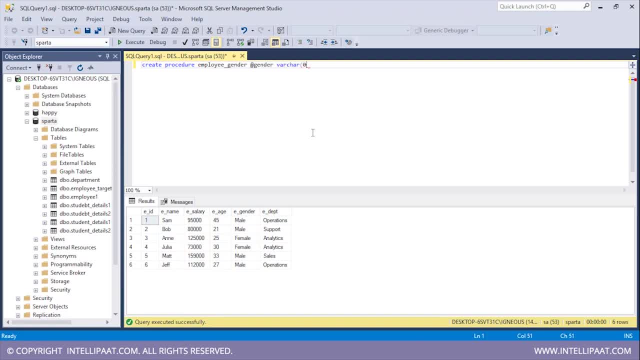 and that is of variable length character with a maximum length of 20.. I will give the as keyword after this and then pass in the statements which would help me to individually access the male employees and the female employees. Select star from the name of the table as employee. I'll follow it up with the. 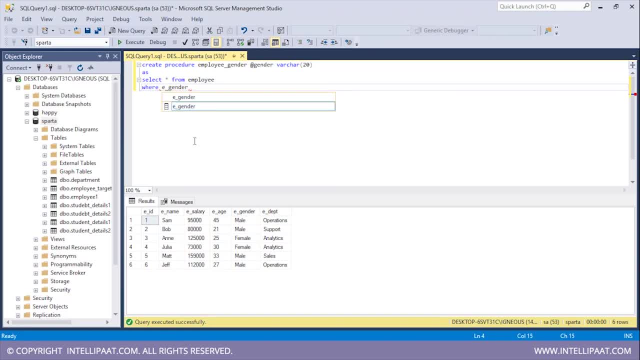 where clause and give the condition. So this time the condition would be: eGender is equal to, at the rate, gender. Now let's understand this properly. So here eGender is basically this column and we are passing in the value of this parameter to this. 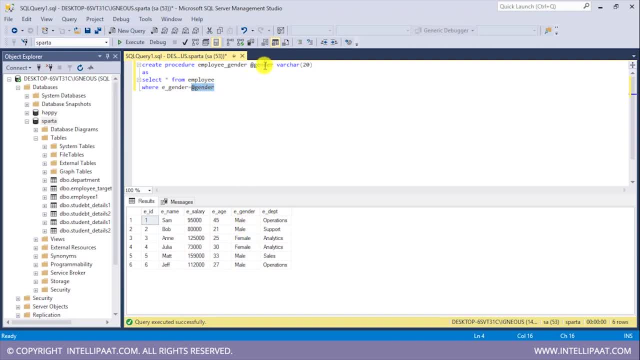 column. So let's say, when we call this procedure and the value is female, then we'll get all of the female employees and similarly, if the value is male, then we'll get all of the male employees. Now let me finish off this procedure with the go keyword. Right, so we have successfully created this employee gender. 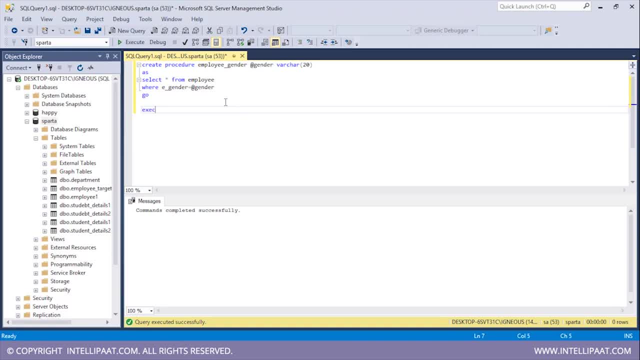 procedure. Now let me go ahead and execute this procedure. So I'll type exec and then give the name of the procedure, which would be employee gender. And now let's say I want all of the male employees, So I will give in the parameter name at the rate gender, and I will give in the value, which would be